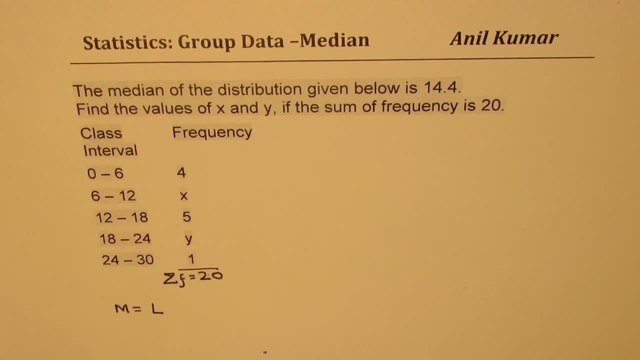 median equals to lower limit of the class interval plus n by 2, the center value the median minus cumulative frequency over the frequency. So that's the formula which we are going to use Now in this particular case. let us first find: 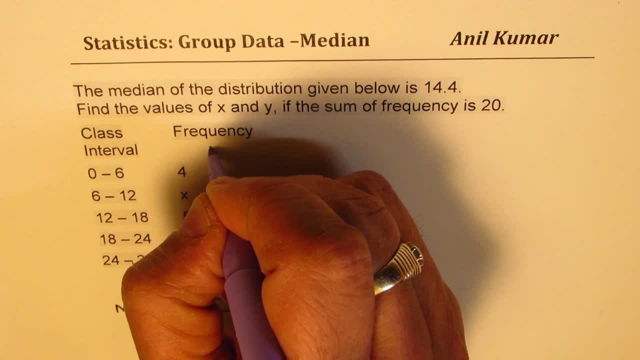 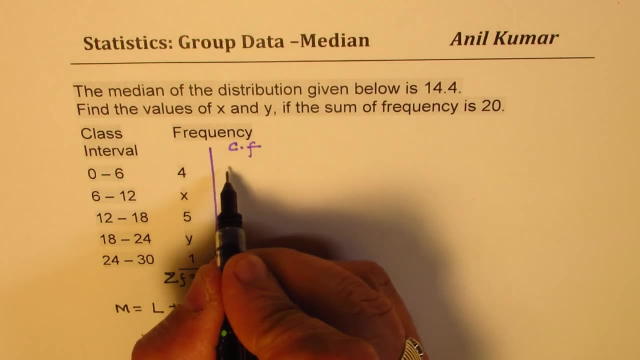 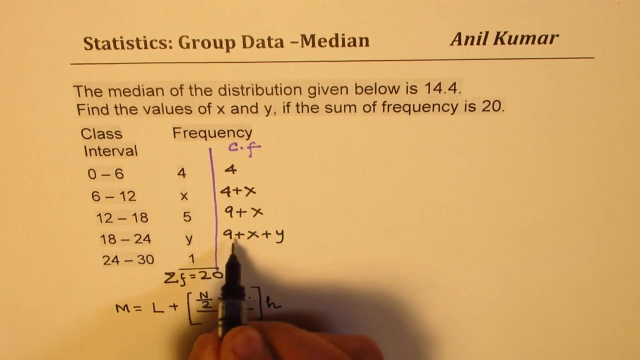 cumulative frequency: right, So let me make an addition column here. I'll just squeeze it in: cumulative frequency 4,. then when you add x, it becomes 4 plus x. Add 5, 9 plus x, add y, it becomes 9 plus x plus y. And when you add 1, it becomes 10 plus x plus y. 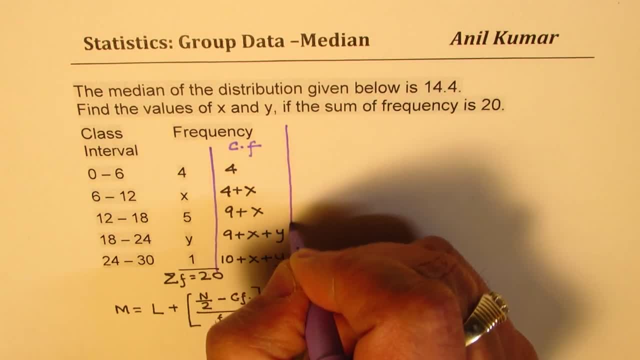 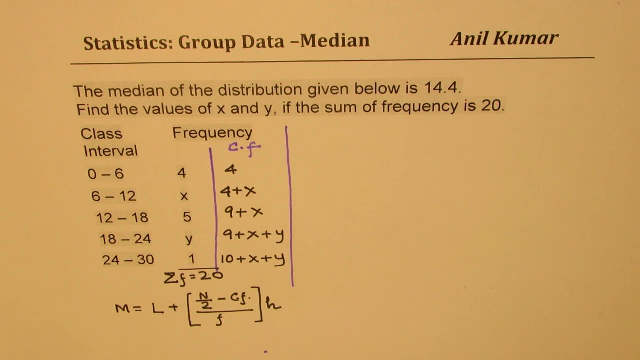 Okay. So when the total is 20, that also tells you one more thing here: that 10 plus x plus y is 20, that means x plus y equals to 10.. Okay, Clear. Now let us try to understand the first statement, Median of the distribution. 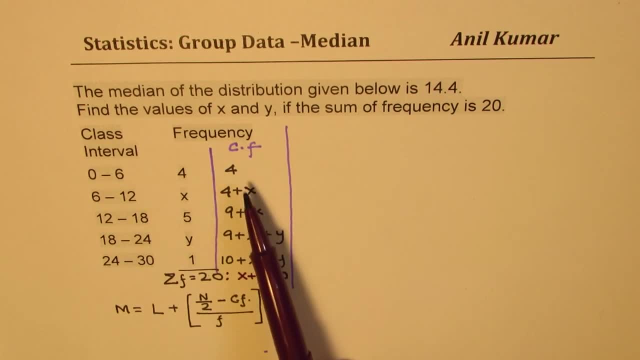 given below is 14.4.. Now, where will be 14.4?? Now, as you can see, x plus y, maximum could be 10.. Even if I take y as 0, x can be 10,, not more than that. So with 10, we can only get a value of 14. here right, Not 14.4.. That clearly, mind Wilde, that is not highest. Now the whole text of this is not too high, right? And if you click here, if youś€ procedure uk and if I gray exercise the, 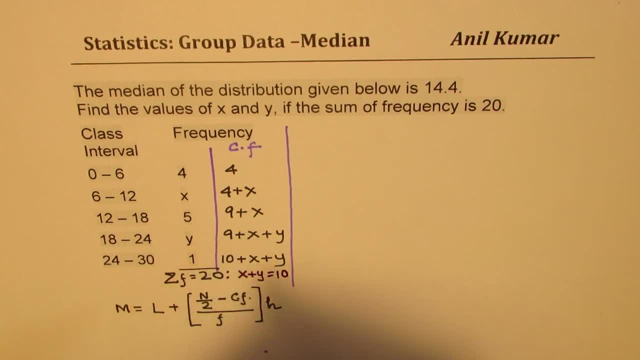 clearly indicates that 14.4 should lie in this particular group. Perfect, because we are assuming it. almost in the center, the group has a frequency of 5. So that becomes our model class correct. So 14.4 will lie in 12 to 18.. Now, in this particular case, 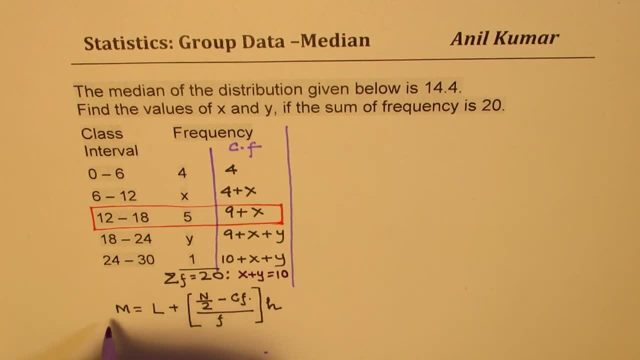 we are already given the median, So we are given median m equal to 14.4.. Now we know all the figures, we can substitute the value and find the unknown right. So here m equals to 14.4, l let us write down what we know. We will write down: m is equal. 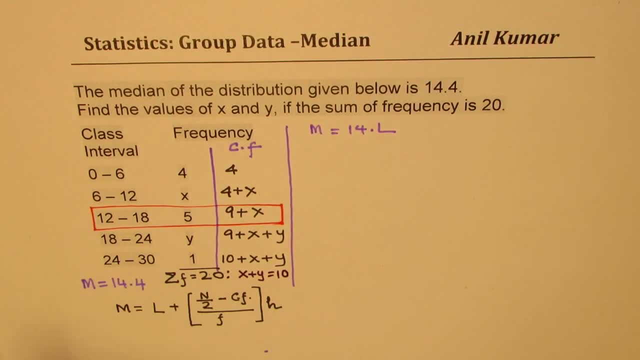 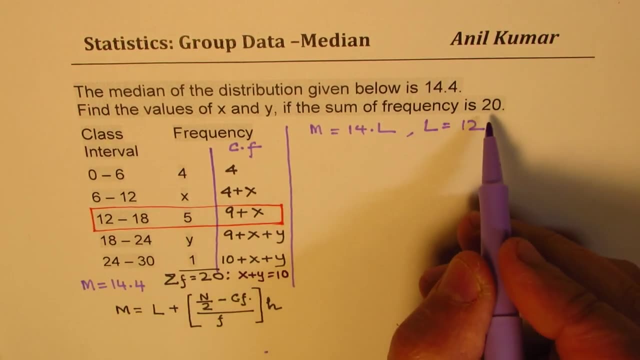 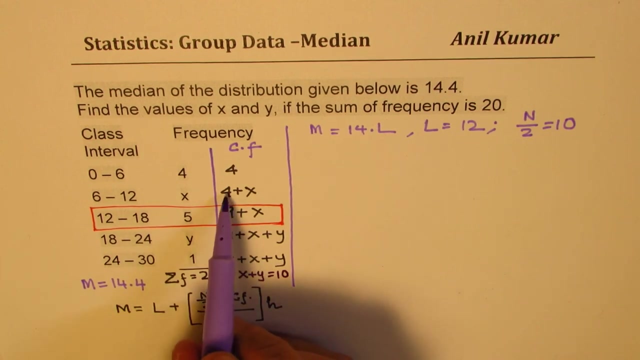 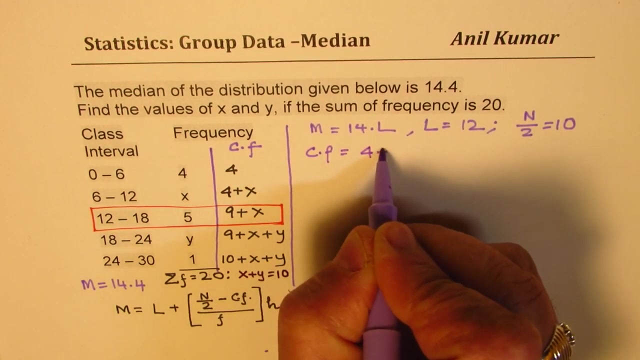 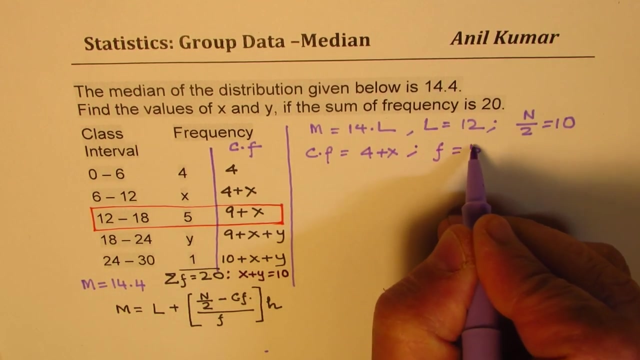 to 14.4. in this formula, Lower l limit is 12, n by 2,. n by 2 is half of 20,, which is 10, right. So n by 2 is 10.. Now we can have the. 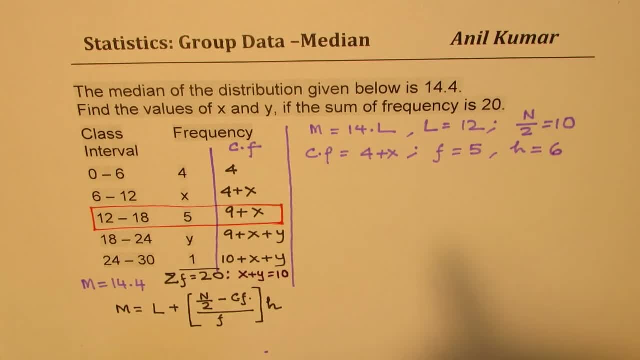 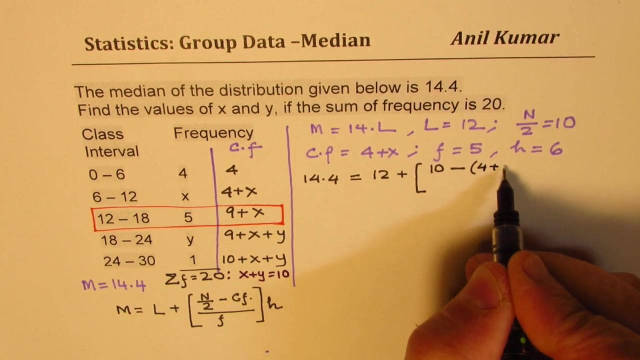 this value 1 plus m, And if we do this gyreshot graph, you can see that the here we have given find the unknown. So we have 14.4 equals 2, 12 plus n by 2 is 10 minus 4 plus x divided. 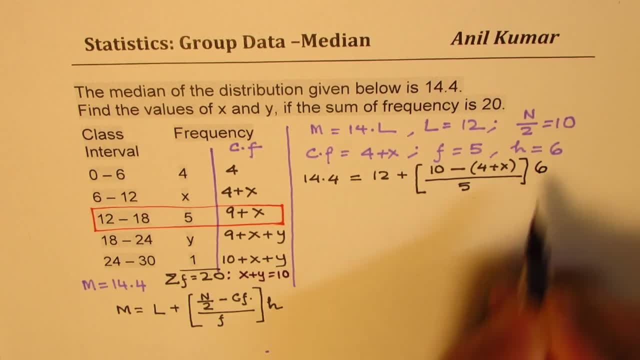 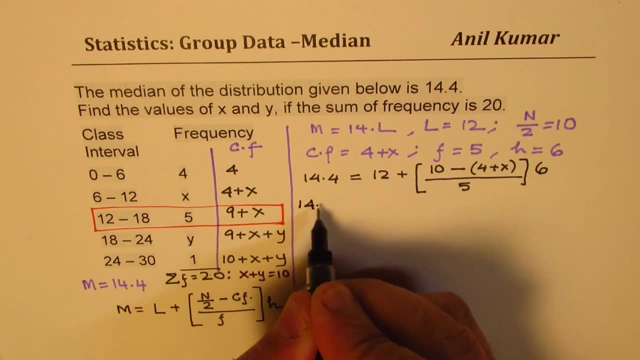 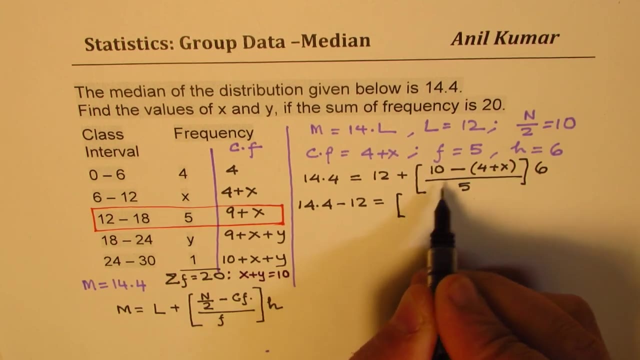 by 5 times 6.. So this can be solved. Let us take 12. on the left side equals 2.. Let us open this bracket: 10 minus 4 is 6, 6 minus x over 5 times 6.. So that gives us 12 point. 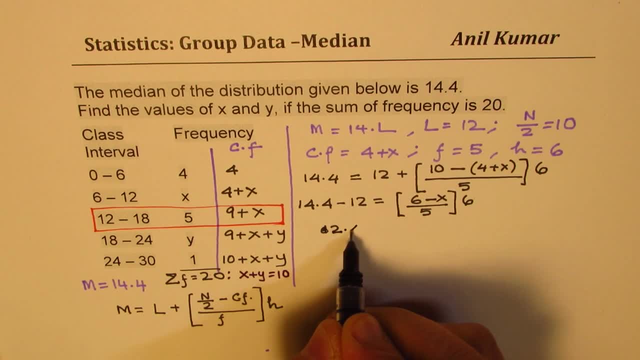 sorry, 2.5.. 2.4 equals to 6 over 5 times 6 minus x. So we get 5 over 6 times 2.4 equals to 6 minus x, correct? So 6 times 4 is 24.. So we get 5 times 0.4 equals to 6 minus x, which is: